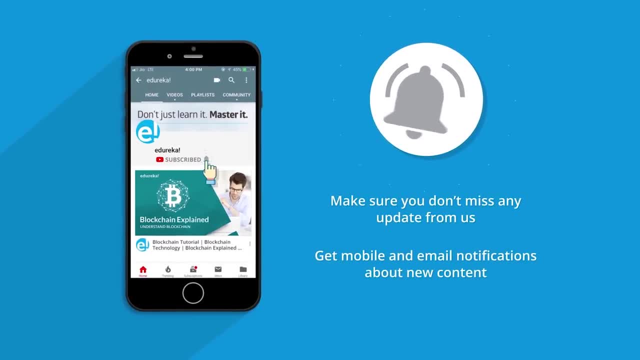 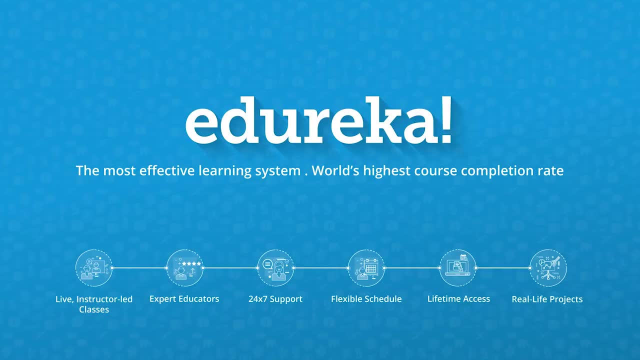 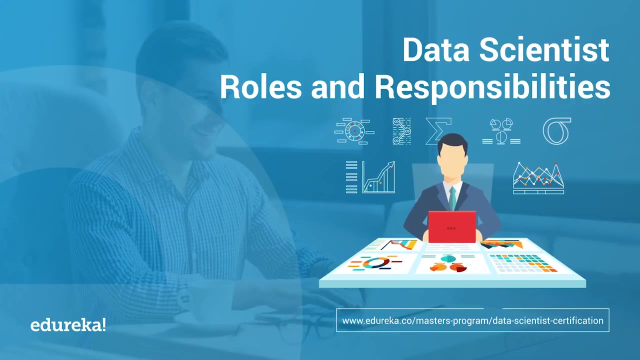 Most organizations have now realized the importance of data-driven decision-making. In the recent year, data science has become inextricable from day-to-day operations. It is employed in products, marketing, engineering and sales to make crucial decisions. Sensational statements of data scientists being the sexiest job has skyrocketed. the 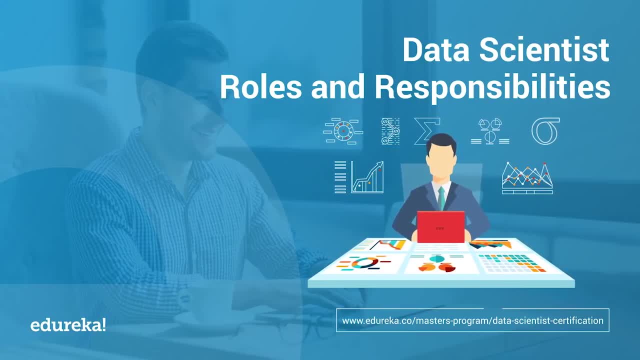 popularity of this nerdy job title. As a result, we can see people flashing their job titles and some striving to become one. Looking at their qualifications, education, experience, aptitude and attitude, isn't it obvious that they don't all fall into the same category? 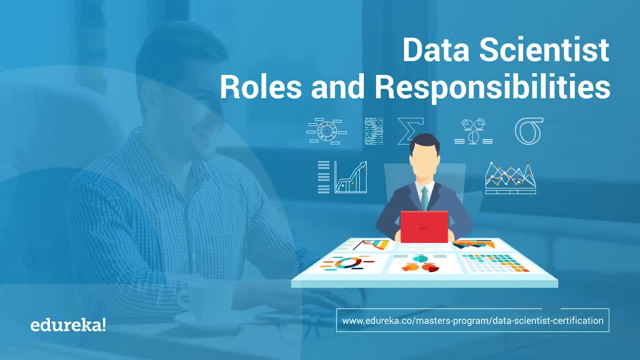 So why are they using the same job title, irrespective of the differences? In this module, we're going to talk about the various roles and responsibilities of different kinds of data scientists, But before we begin, let's talk a little bit about what you should. 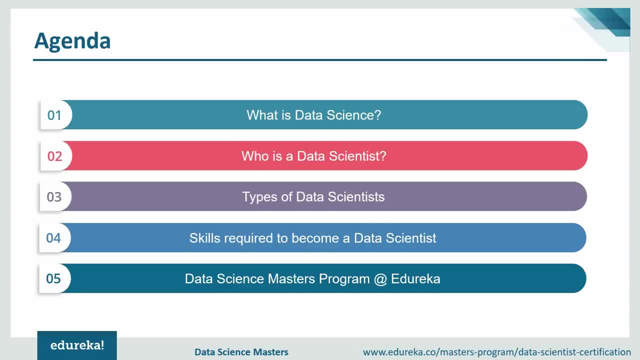 expect from this session. So first of all, I'll be giving you a little brief about what data science is and who is a data scientist, the basic roles and responsibilities, the company's hiring and some market stats. Then we'll be going in-depth about different types of data scientists. 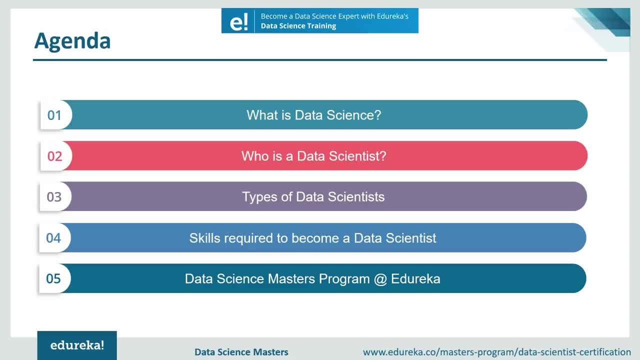 and the skills required and the job descriptions regarding them. Then we are going to boil down to some basic skills you require to enter the data science domain And finally, we're going to talk about the data science master's program at Edureka. So, without much ado, let's go straight into the module. 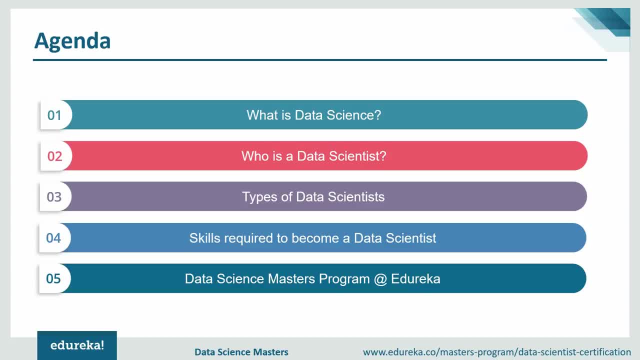 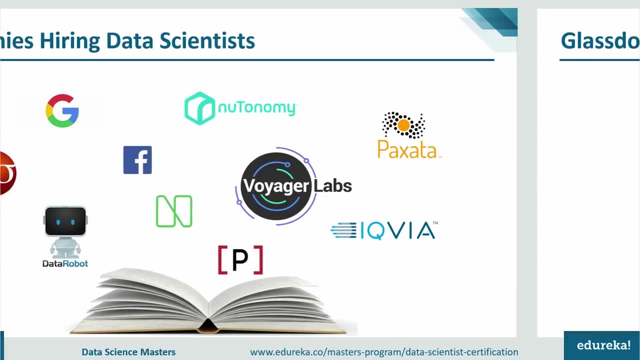 Now data scientists are sought after. some of the biggest names in business, in the lines of Google, Facebook and Amazon, all willing to pay hefty salaries to skill-certified data scientists. This is precisely why Glassdoor has ranked it number one in the list of best jobs. 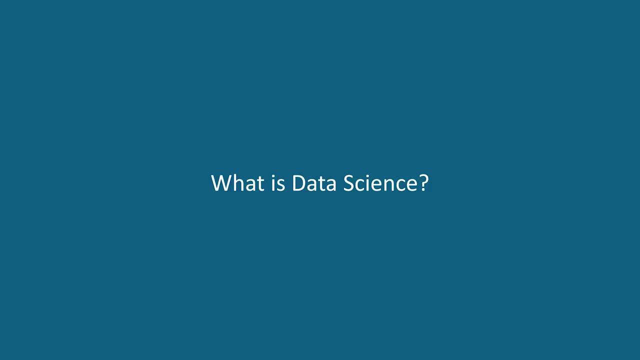 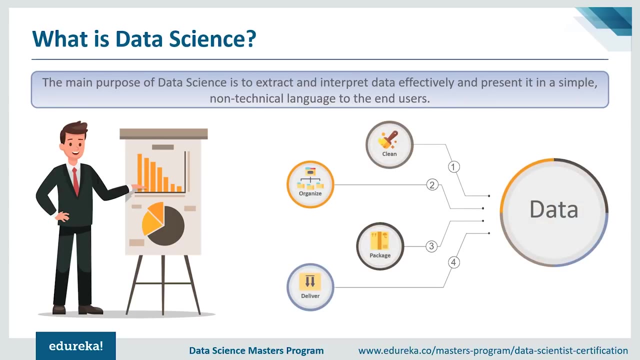 and the demand for data scientists has never been greater. But what is data science Now? data science is an umbrella term that encompasses data analytics, data mining, artificial intelligence, machine learning and several other related disciplines. Now data science mainly consists of four components, that is, cleaning, organizing, 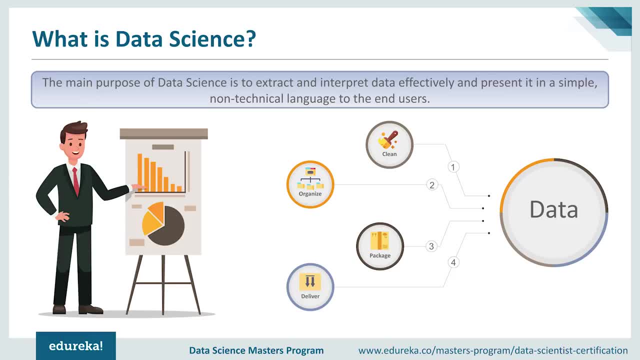 packaging and delivering data. So let's have a brief look into these Now. cleaning and organizing data is where the planning and execution of the physical and emotional work is done. So the planning and execution of the physical and emotional work is done, And the planning and 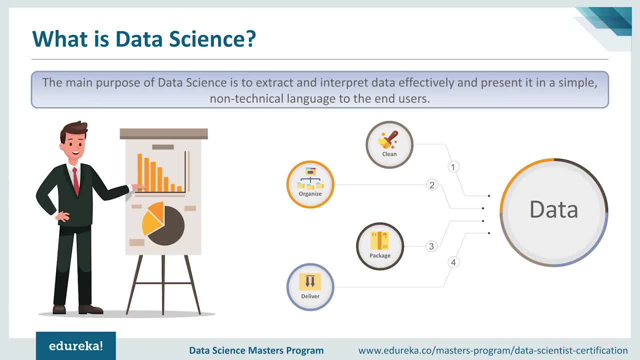 organization of the physical and emotional work is done, So the planning and organization of the physical storage and structure of the data takes place After applying the best practices. it is termed as data handling. Now, packaging the data is where prototypes are created, The statistics is applied. 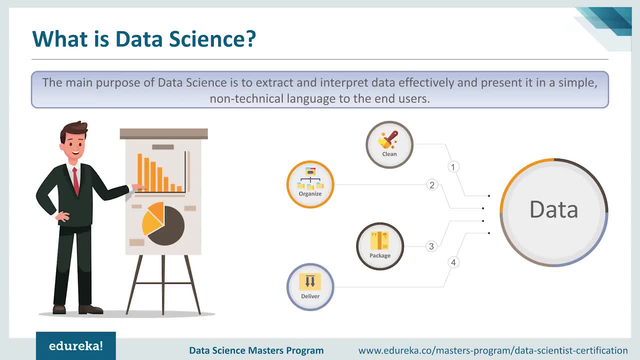 and the visualization is developed. It involves logically as well as aesthetically, modifying and combining the data in a presentable form. Finally, we have delivering the data. Delivery is where the story is narrated and the value is received. It makes sure that the final outcome has been 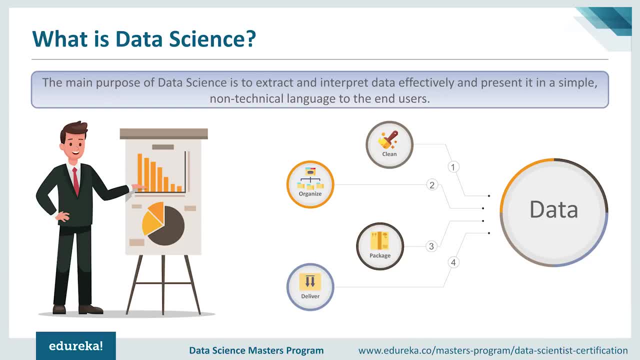 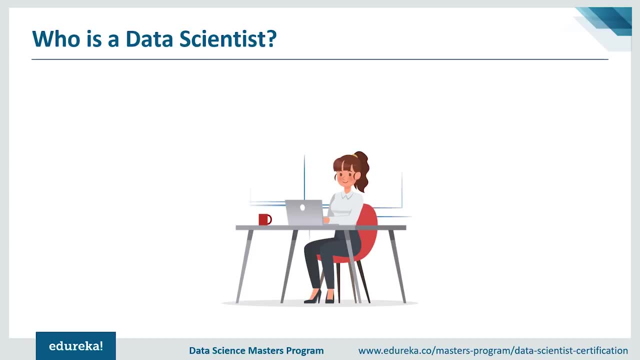 delivered to the concerned people. But who takes care of all this? The answer is obvious: It's a data scientist. Now, the role of a data scientist is indeed a challenging one, Though the skill sets and competencies that data scientists employ differ extensively to be an efficient data. 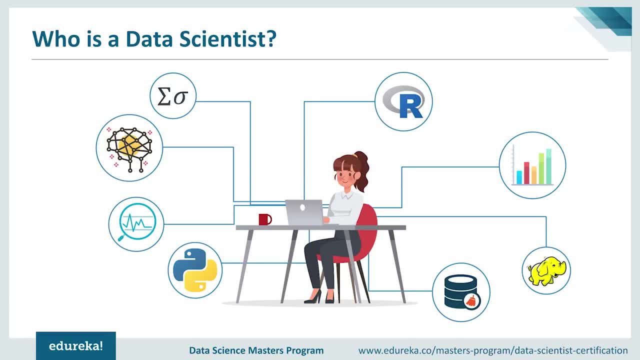 scientist. one should be very innovative and distinct in his approach in applying various techniques intelligently to extract data and get useful insights in solving business problems and challenges. They must be well-versed in statistics and mostly have a math-heavy background. They must have the ability to locate and construe rich data resources, have a hands-on experience in R. 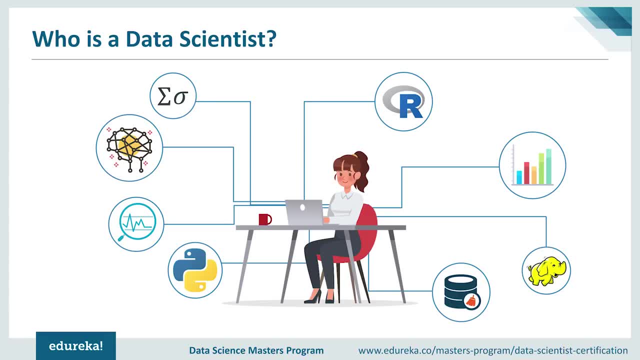 or Python, or preferably both, perform data conditioning, that is, converting data into a useful form by applying statistical and math tools and predictive analysis, and finally have an idea about managing large amounts of data, so basically, some big data. Apart from this, being a team leader and communicating effectively is a certain plus. This 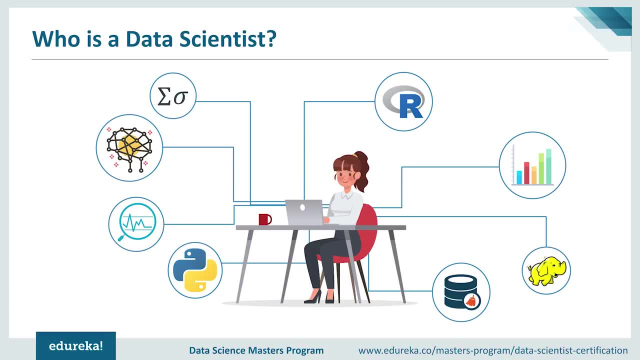 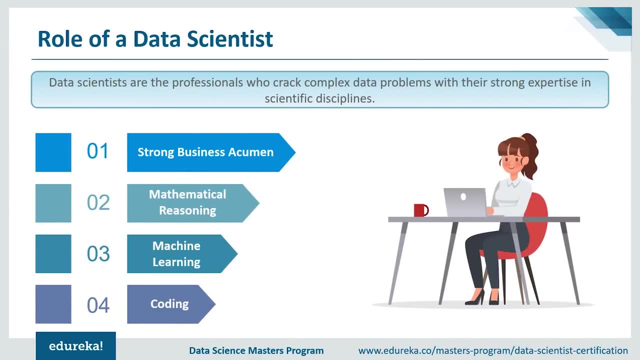 helps them to deliver precisely to other business analysts, product managers and engineers. In brief, a data scientist should be very strong in any of these skills or all. They must have a really strong business acumen, strong statistical reasoning, a working knowledge of machine. 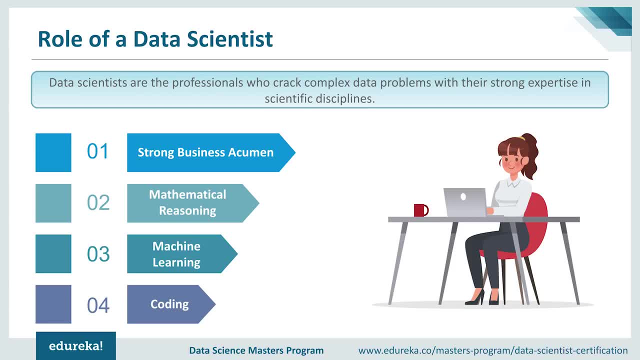 learning and coding in either R or Python, or both. For instance, a person with a strong statistics background can become a data scientist, while acquiring substantial skills in coding in business. As a data scientist, you'll basically be responsible for jobs that span three domains of skills: statistical. 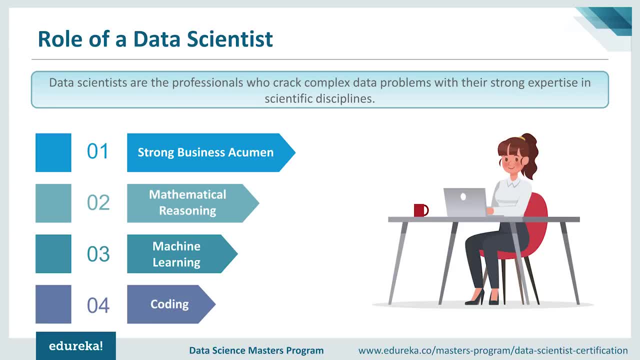 reasoning, business communication or leadership and programming. You'll often be tasked with leading data science projects from end to end. So, basically, a data scientist is like a webmaster, who not only needs to be a jack-of-all-trades, but has a job that needs to solve a lot of problems. The fact that you're a data scientist is like a webmaster, who not only needs to be a jack-of-all-trades, but a data scientist is somehow capable of doing all the work that you do. You learn the skills you need. You. 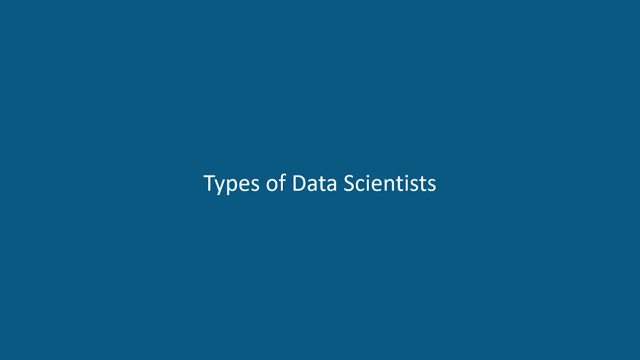 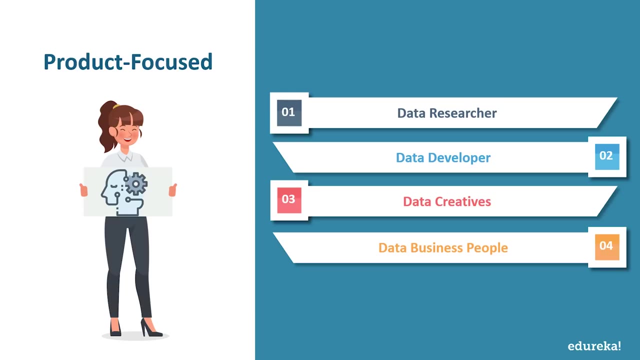 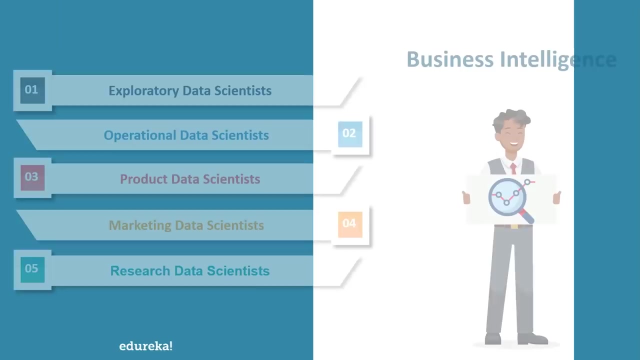 but also a master of at least one of these fields. This is probably the reason why data scientists can be broadly classified into two main categories. One is the product-focused data science. This basically involves analyzing the analyzers. And two, you have the business intelligence side of data science. 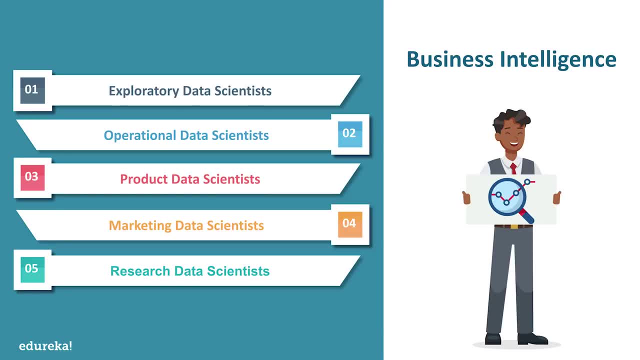 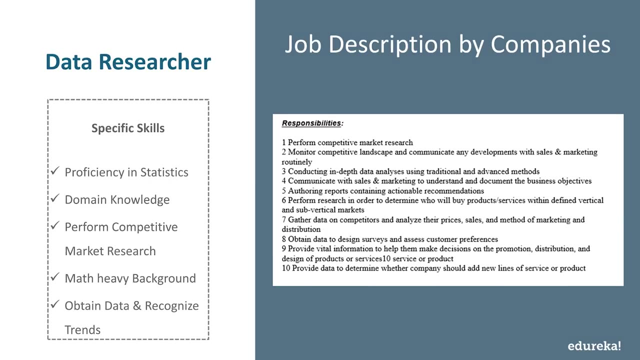 These are the ones which represent the business side and are responsible for making vital decisions through data analytics techniques. There are a few categories in each of them, which we shall be discussing in detail soon after, So let's start with a data researcher Now. professionals in this category come from the academic world. 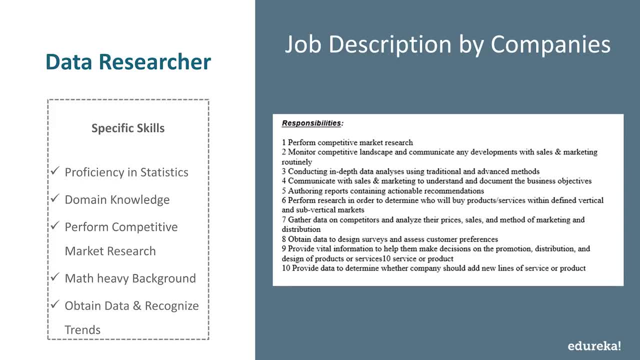 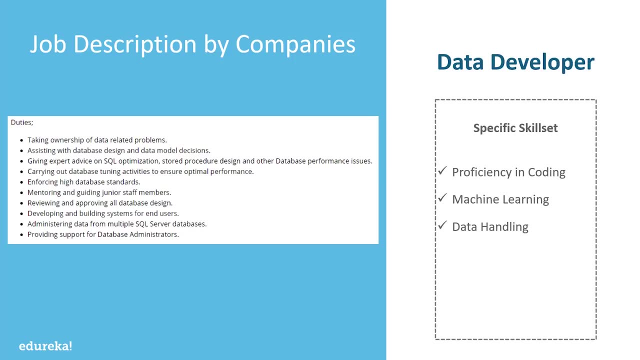 and have in-depth backgrounds in statistic or the physical and social sciences. This type of data scientist often holds a PhD, but is weakly skilled in machine learning, programming or business. Next we have data developer. These guys tend to concentrate on the technical issues that come with handling data. 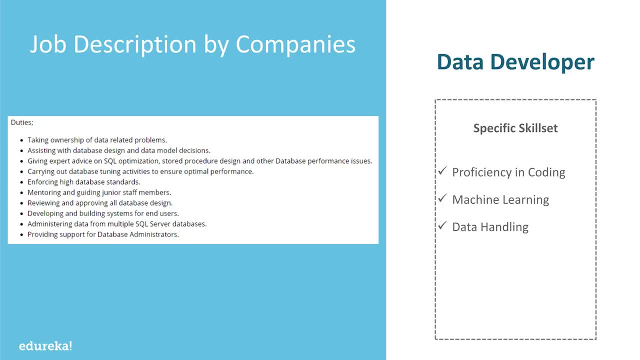 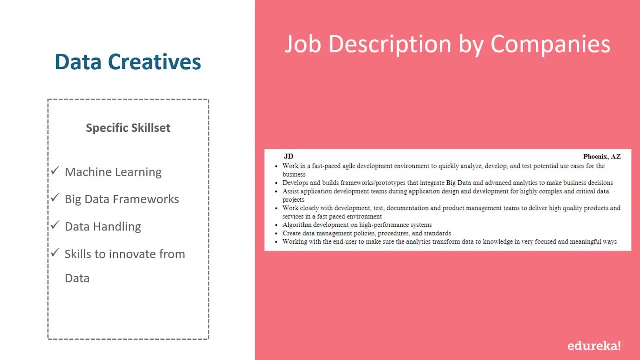 They're strong in programming in R or Python and machine learning, but weak in business and statistics skills. Next, we have data creatives. These are the guys who make something innovative out of mountains and mountains of data. They are strongly skilled in machine learning, big data programming. 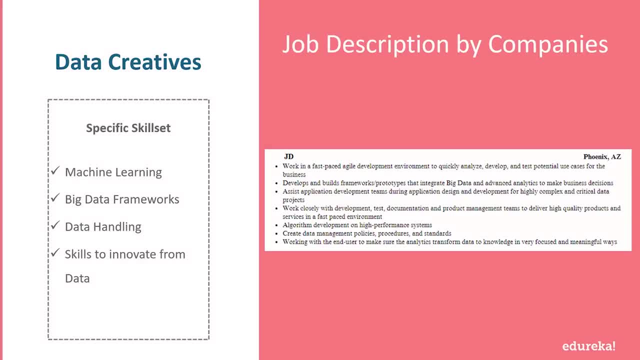 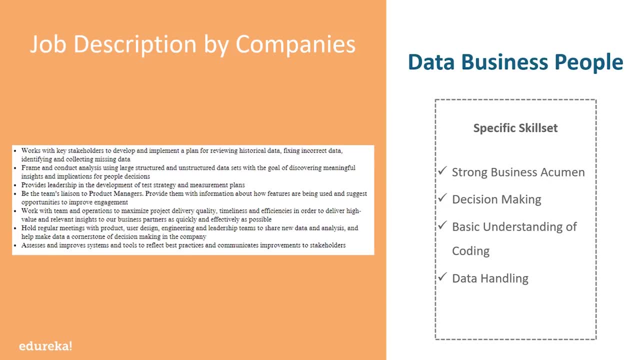 and other skills to handle massive amount of data. Next, we have data business people. They represent a business side and are responsible for making vital business decisions through data analytics techniques. Now, they are an eclectic blend of business and technical proficiency. Now let's talk a little bit about BI-based data scientists. 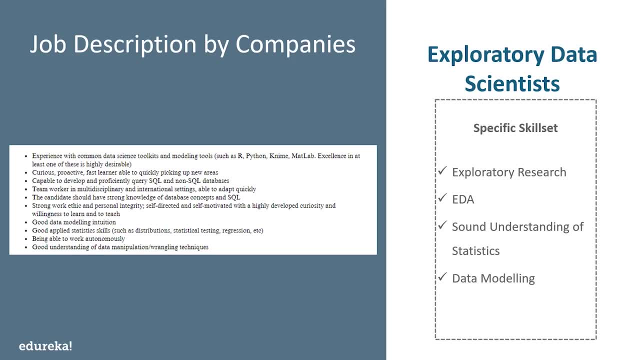 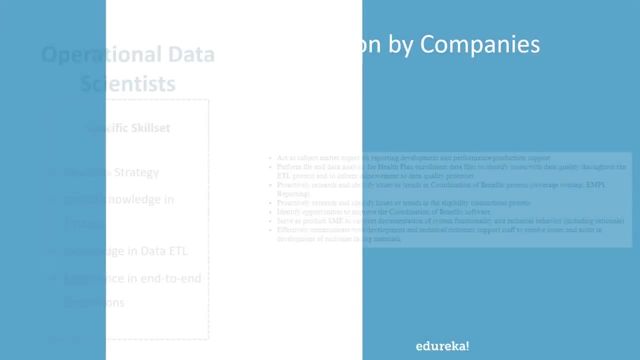 First of all, we have quantitative or exploratory data scientists. Now these are the ones that are inclined to have PhDs and use theory to comprehend behavior. By combining theory and exploratory research, these data scientists improve products. Next, we have operational data scientists. 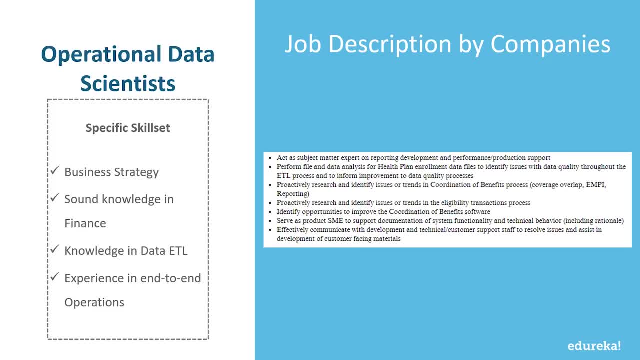 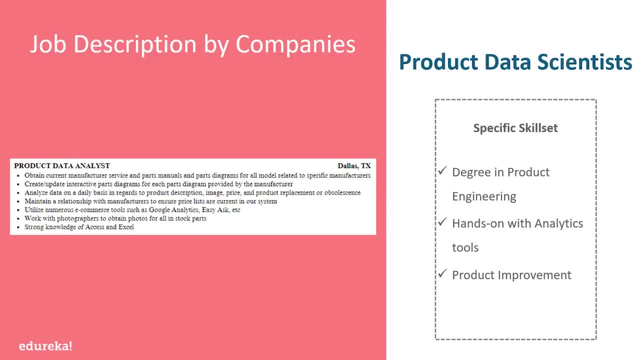 Next we have product data scientists. Now product data scientists fit into the product management or engineering form of data science. Their job is to sift through logs and analysis tools to understand the way users make use of a product and make use of it. They also make use of that knowledge to fine tune this product. 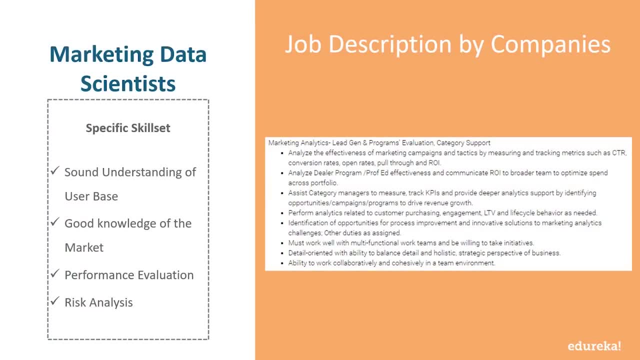 Next we have marketing data scientists. Now, marketing data scientists focus on the user base. They evaluate performance and work on improving efficiency. So pretty much like the standard marketing guy, but in data science. And finally we have the research data scientists. 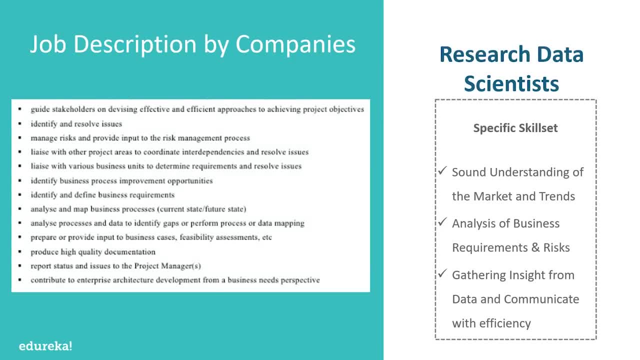 Now these data scientists create insights from a data set. It's rare for startup companies to employ research scientists because the output isn't tied to profits, But larger company think tanks and financial institutions definitely have a spot for these data scientists. Now, this classification shows that any bunch of people 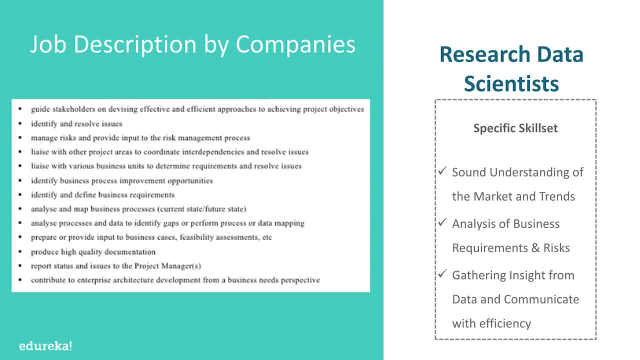 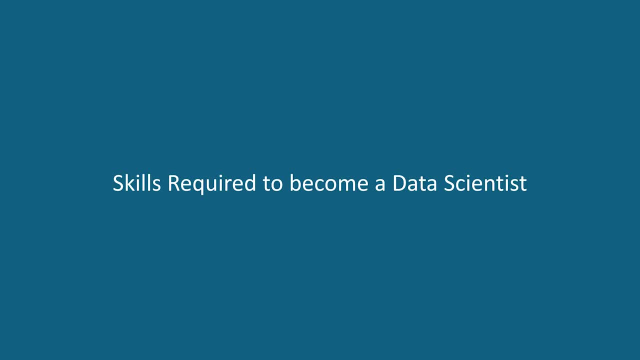 can be put in any one category and the right type of data scientist can be chosen based on the organization's requirement. So before choosing the type of data scientist you want to become, consider the skills required, or the skills you already possess, to proceed in the appropriate direction. 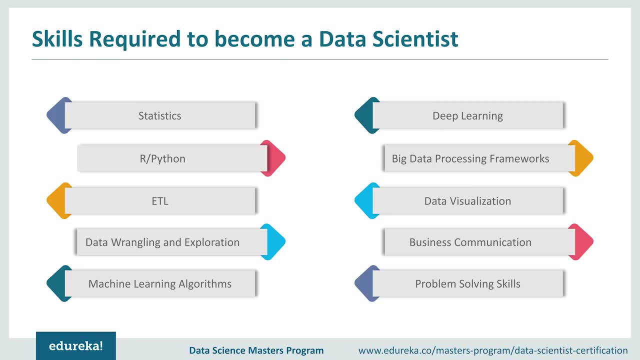 It all boils down to these basic skills which you need if you want to enter the data science domain. First of all, we have statistics Now. Wikipedia defines it as the study of, collection, analysis, interpretation and presentation of data. Therefore, it shouldn't be a surprise that data scientists 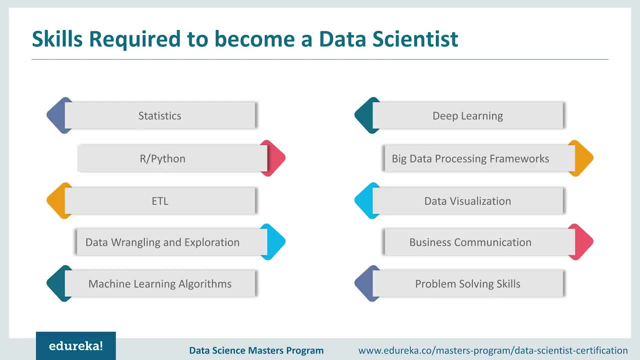 need to know statistics, For example, data analysis requires descriptive statistics and probability theory at a minimum. These concepts will help you make better business decisions from data sets. Next we have programming languages. With programming languages, you can manipulate the data and apply certain algorithms. 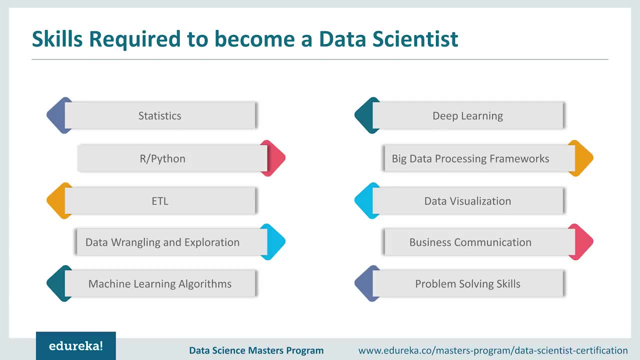 to come up with some meaningful insights. Now. Python and R are the most widely used languages by data scientists. The primary reason is the number of packages available for numeric and scientific computing With the help of these packages, like SkilletLearn in Python and E1071 and Rpart in R. 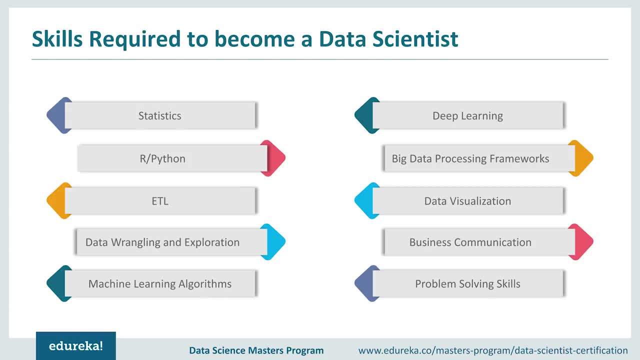 it becomes really easy to apply machine learning algorithms. Next, we have data extraction, transformation and loading. It is commonly known as ETL. Suppose we have multiple data sources like MySQL, DB, MongoDB, Google Analytics, etc. You have to extract the data from such sources. 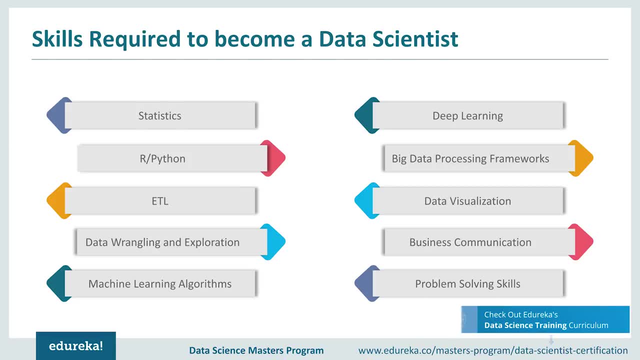 and then transform it for storing in a proper format or structure for purposes of querying and analysis. Finally, you have to load the data in the data warehouse where you will be analyzing the data. So for people from ETL, data science can be a good career option. 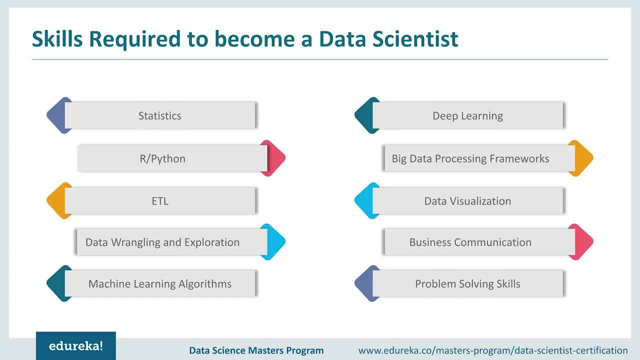 Next we have data wrangling and data exploration. Now you have data in the warehouse, but that data is pretty inconsistent, So you have to clean and unify the messy and complex data sets for easy access and analysis. This is termed as data wrangling. 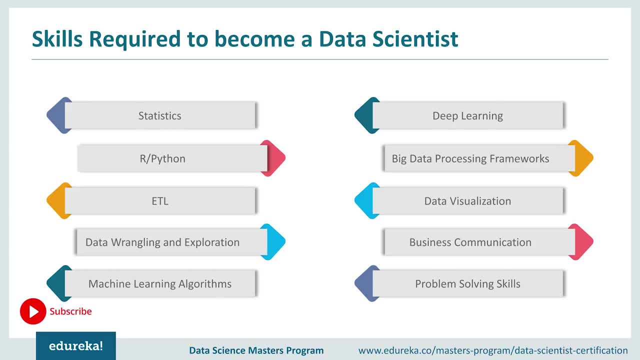 Exploratory data analysis, or EDA, is the first step in your data analysis process. Here you make sense of data that you have and then figure out what questions you want to ask and how you want to frame them, as well as how is it best. 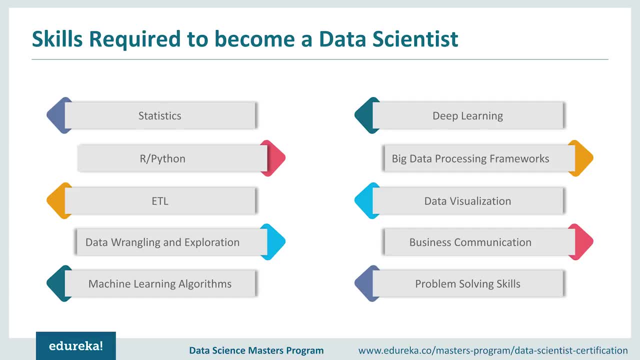 to manipulate your available data sources to get the answers you need. You do this by taking a broad look at patterns, trends, outliers and unexpected results and accomplish your task. Next we have machine learning and advanced machine learning, which is also known as deep learning. 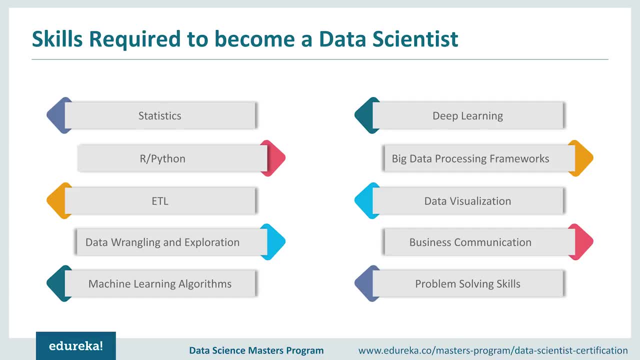 Now machine learning, as the name suggests, is the process of making machines more intelligent that have the power to think, analyze and make decisions. by building precise machine learning, models and organization has a better chance of identifying profitable opportunities or avoiding unknown risks. You shall have a good hands-on knowledge of various supervised 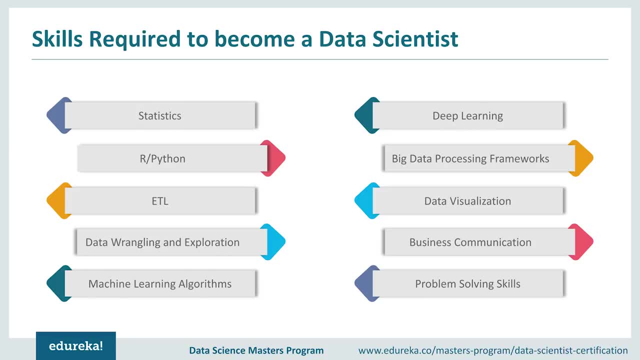 and unsupervised algorithm if you want to become a data scientist tending to this field. Next, we have deep learning, which has taken the traditional machine learning approach to a next level. It is inspired by the biological neurons, or what you call brain cells. 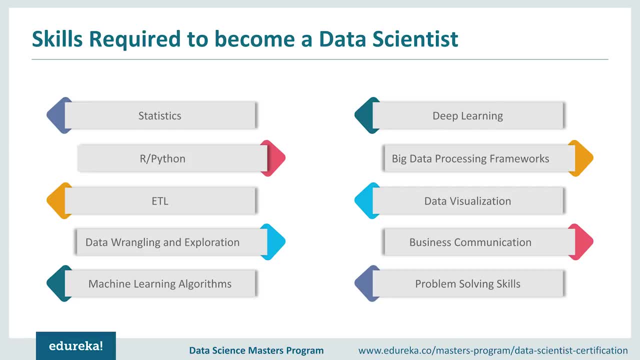 The idea here is to mimic the human brain. a large network of such artificial neurons is used, and most organizations these days ask for knowledge in deep learning, So it is advisable to not miss this. next, We have big data processing frameworks now a huge amount. 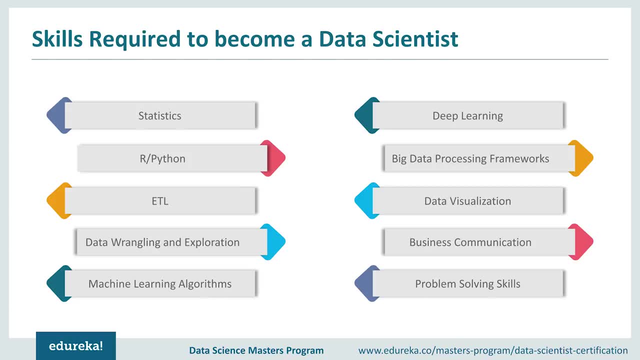 of data is required to train machine learning or deep learning models. earlier, because of the lack of data and computational power, creating precise machine learning or deep learning models was not possible. nowadays, huge amounts of data is generated at a good velocity. This data can be structured or unstructured. therefore, it cannot be processed. 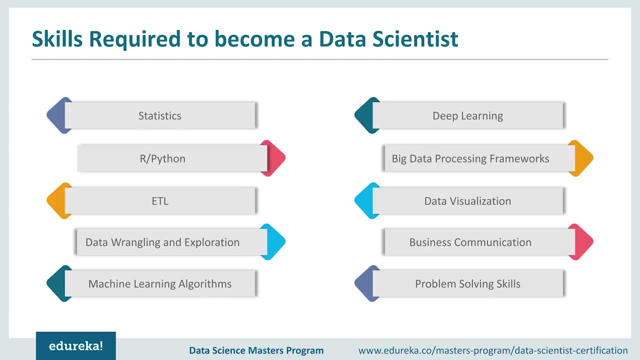 by traditional data processing systems. such humongous data sets are termed as big data. Therefore, we require the frameworks like Hadoop and spark to handle big data. nowadays, Most of the organizations are using big data analytics to gain hidden business insights. It is therefore a must-have skill for a data scientist. 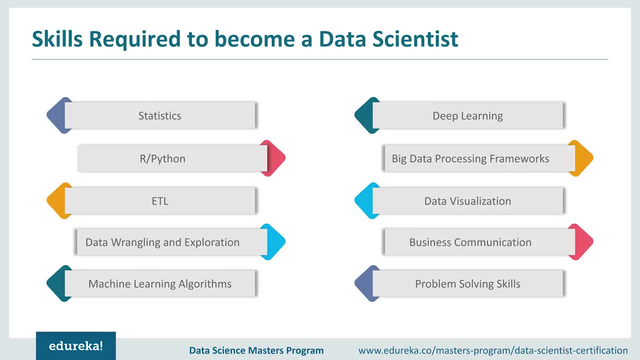 Then we have data visualization. now, data visualization is one of the most important parts of data science, and it has always been. you have to present the data in an understandable and visually appealing format. Data visualization is one of those skills that data scientists have to master in order to communicate better to end users. 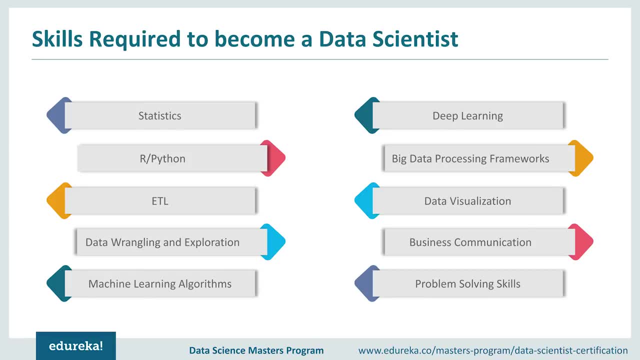 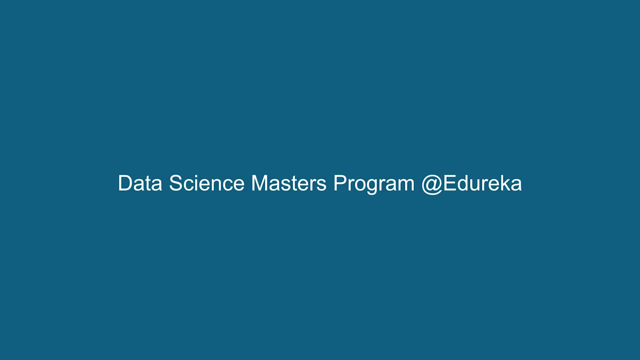 There are multiple tools like tableau and power bi, which give you a nice, intuitive interface. apart from all the data scientist skills that I have mentioned right now, You must also possess a data-driven problem-solving approach, and this will only come with experience. your journey to becoming a data scientist is definitely going to be pretty long. 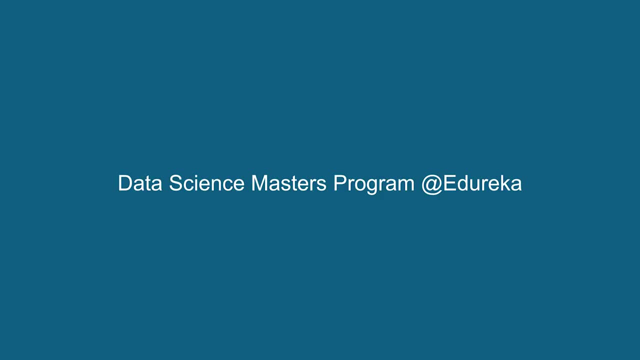 And I know as a working professional- It is very difficult to devote time to learning something new, and that's why it is always recommended to go for an online training. The time is ripe to upskill in data science and to take advantage of the data science career opportunities. 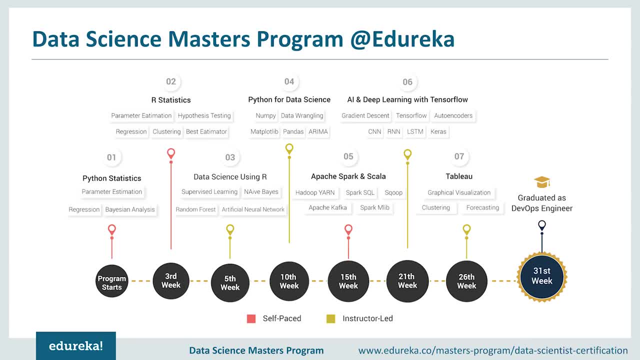 that come in your way. at Edureka, You can learn at your own pace and at your own time from the very location of your choice. but the experience here is much more than this and caters to every single aspect of a data scientist skill development. 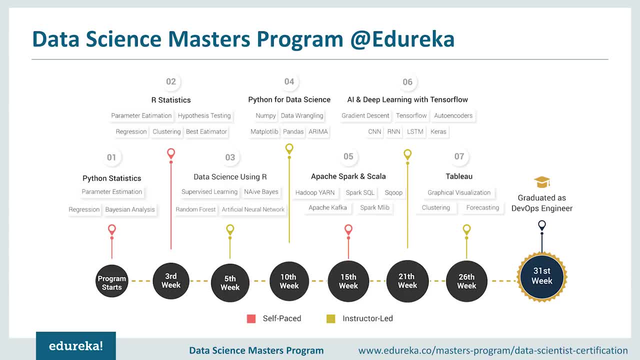 We have a specially curated data science Masters program which helps you gain expertise in machine learning. Python are, and a bunch of different visualization tools. You learn concepts of statistics, time series, text mining and get an introduction to deep learning as well. So who are you going to be? a programmer, a statistician?